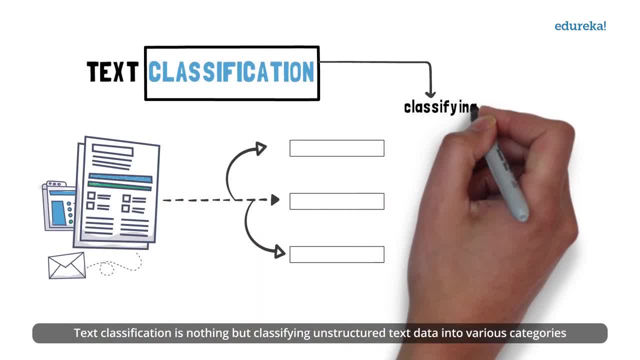 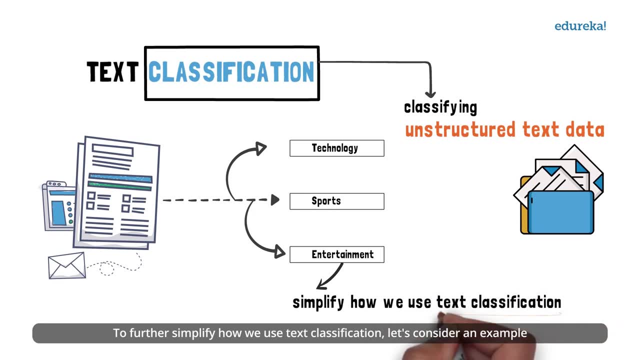 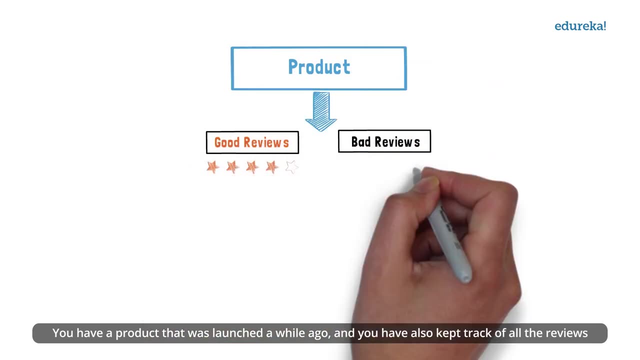 advantage. Text classification is nothing but classifying unstructured text data into various categories. To further simplify how we use text classification, let's consider an example. You have a product that was launched a while ago and you have also kept track of all the reviews that the product got on all the platforms across the internet. 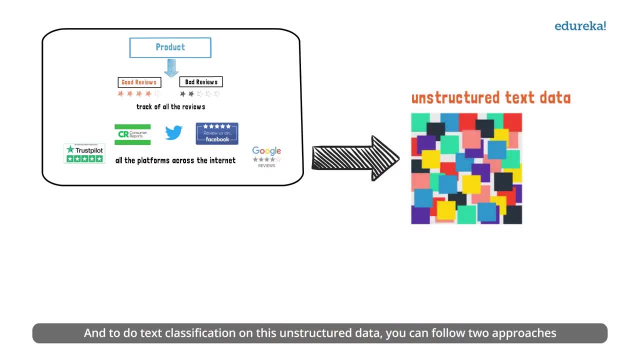 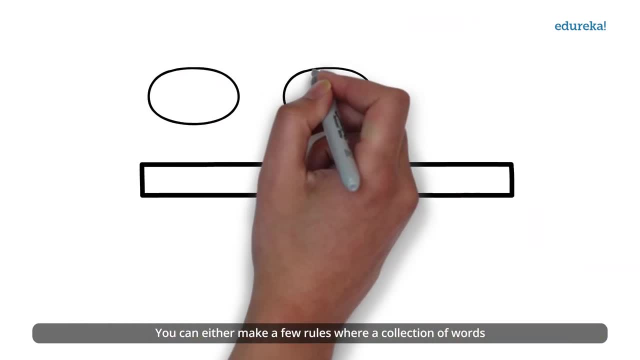 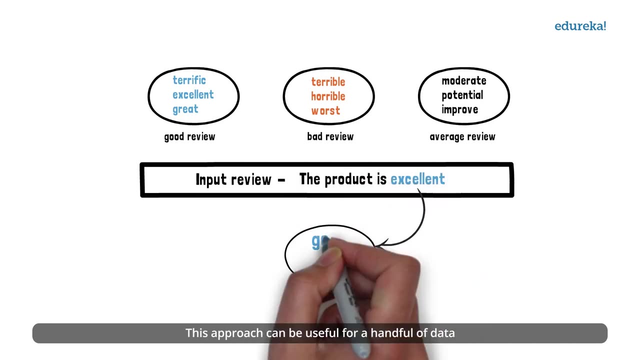 Now what you have is unstructured text data, And to do text classification on this unstructured data you can follow two approaches. One: you can either make a few rules where a collection of words will decide the sentiment of the input text. This approach can be useful for 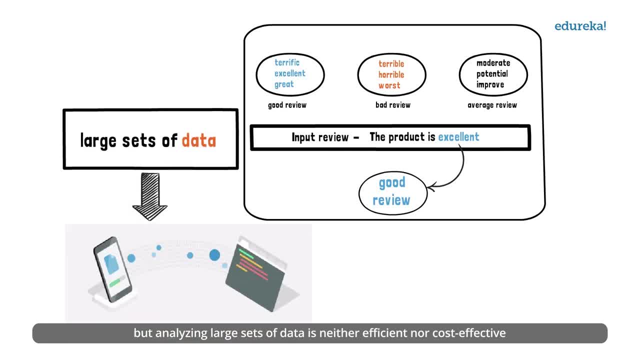 a handful of data, but analyzing large sets of data is neither efficient nor efficient. So in this case, you can either create a statement or you can write the sentence, or you can write the sentence. Either way, you can create a statement or you can create. 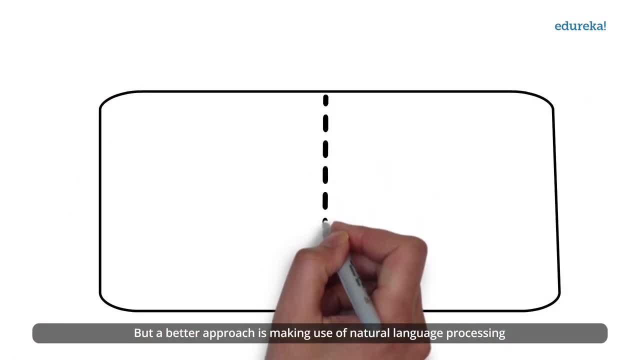 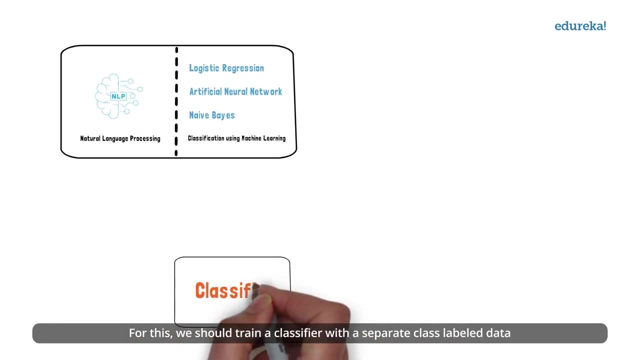 a statement or you can write the sentence, or you can write the sentence or you can write a statement. nor cost effective, But a better approach is making use of natural language processing and classification using machine learning. For this we should train a classifier with. 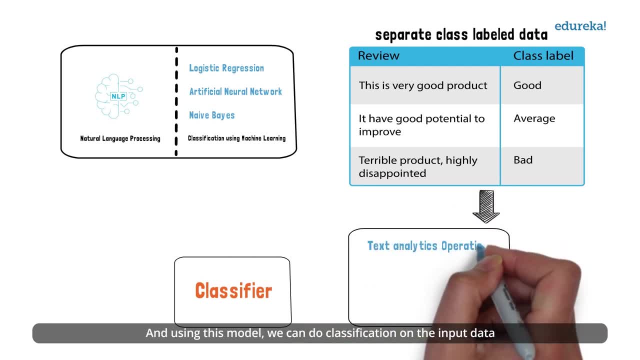 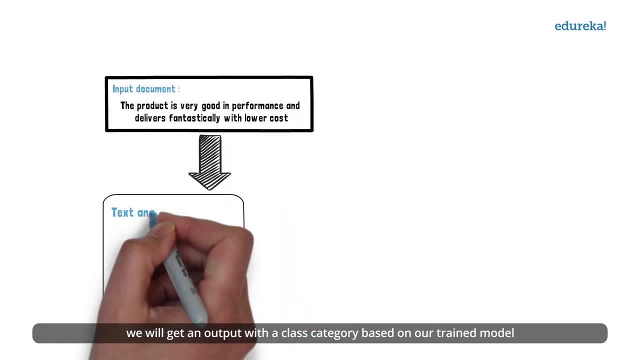 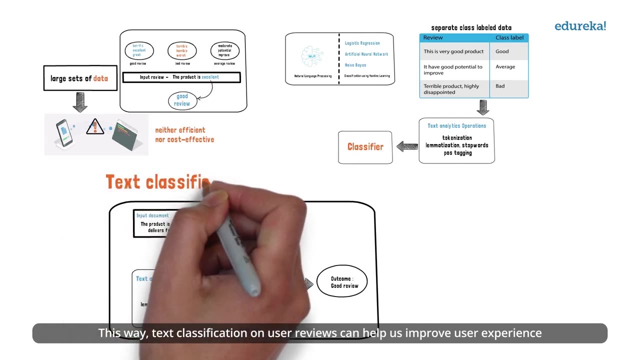 a separate class labeled data and using this model, we can do classification on the input data. When we give input to the classifier, we will get an output with the class category based on our trained model, telling us if the review is bad, average or good. This way text classification. 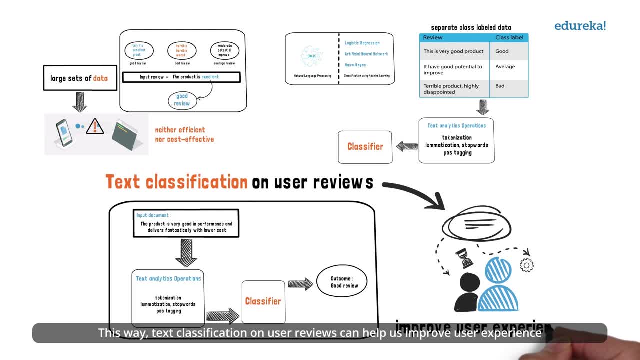 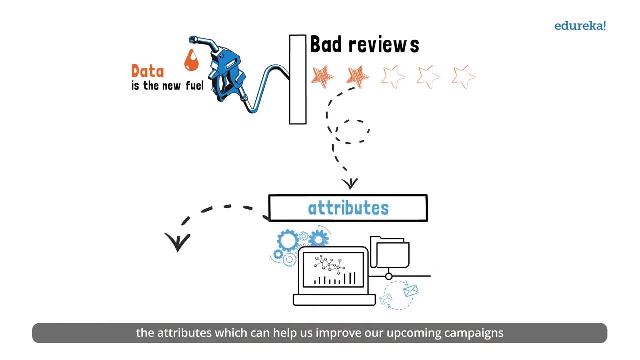 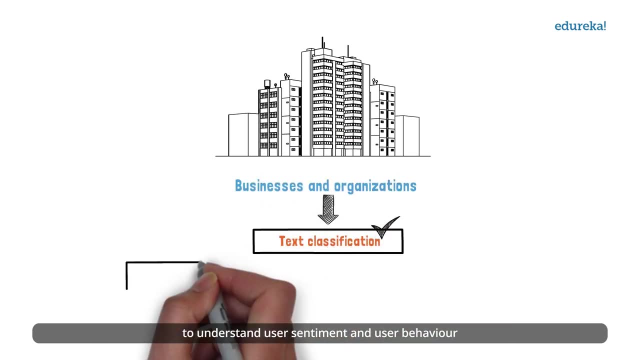 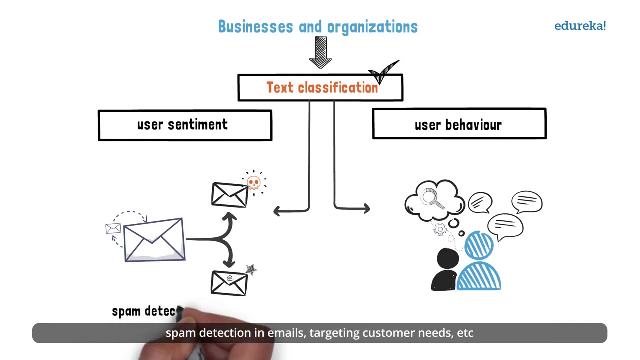 on user reviews can help us improve user experience. Data is the new fuel. This- even bad reviews- can help us identify the attributes which can help us improve our upcoming campaigns. Businesses and organizations are following this trend to understand user sentiment and user behavior. Text classification can also be used for applications like spam detection in 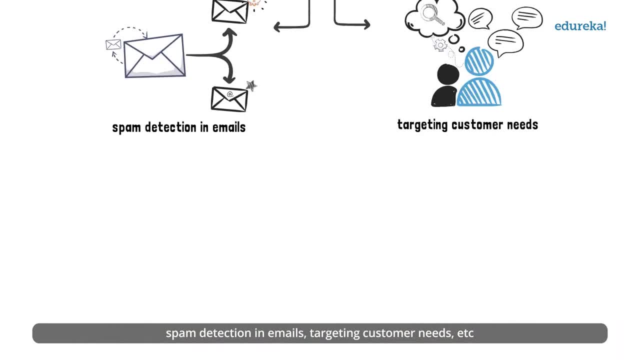 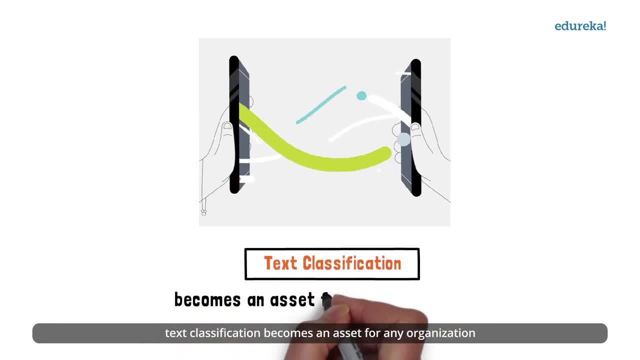 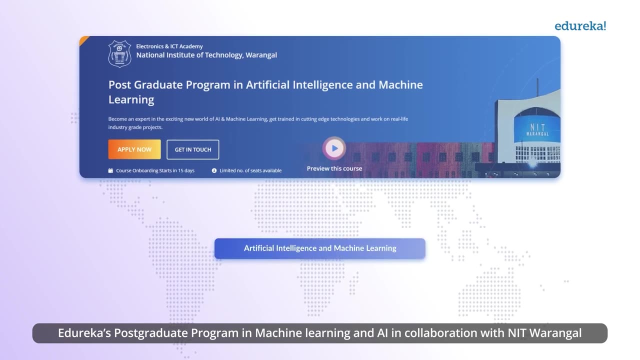 emails targeting customer needs, etc. In this DNA, where data is generated every second of the day, text classification becomes an asset for any organization. Edureka's postgraduate program in machine learning and artificial intelligence, in collaboration with NIT Varangal, can help you learn text classification and natural language. 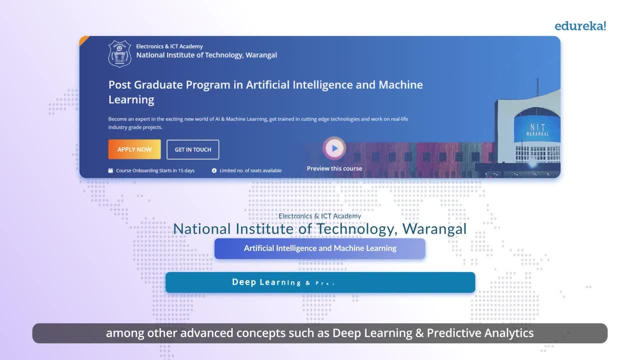 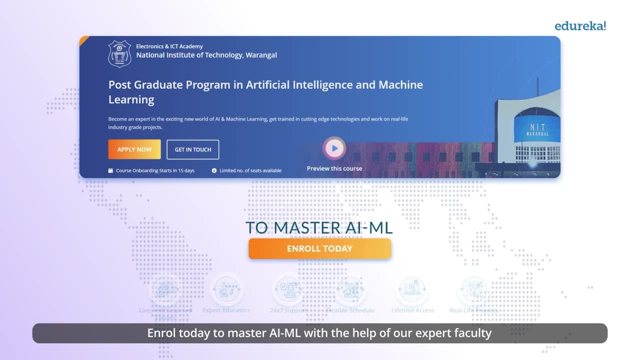 processing, among other advanced concepts such as deep learning and predictive analytics. Enroll today to master artificial intelligence and machine learning with the help of our experts. Learn more at edurekaedu.